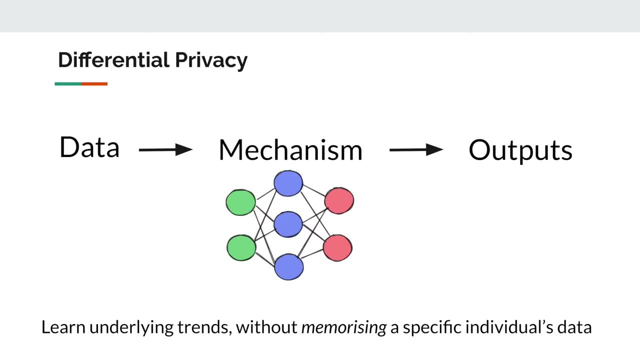 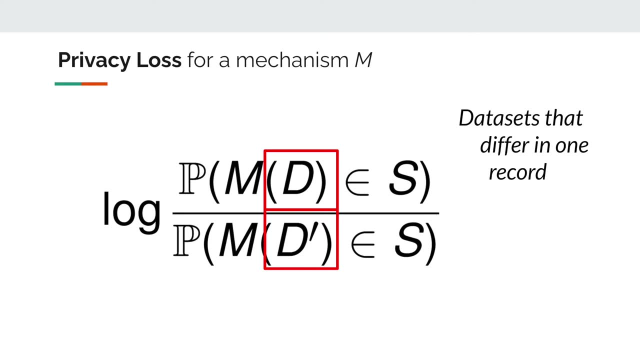 individual's data. We measure this in our differential privacy definition by considering a single user's data, We bound the amount the mechanism's outputs change, which we define as this log of the ratio of the two probabilities. The bound, epsilon, is called our privacy budget. 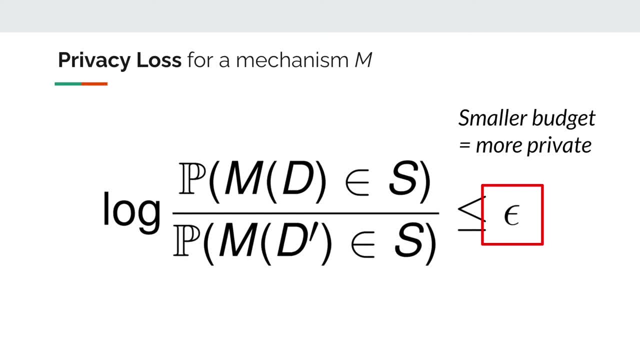 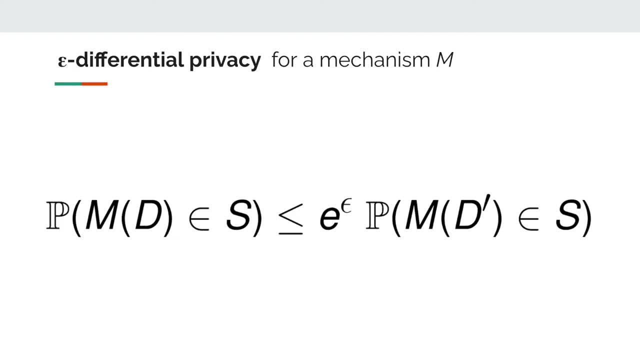 and if it holds for all data sets D and D prime, whatever the outcomes. S we say that the mechanism is epsilon differentially private. In practice we rearrange this as follows: This epsilon bound is really tight and is hard to guarantee for all outcomes. 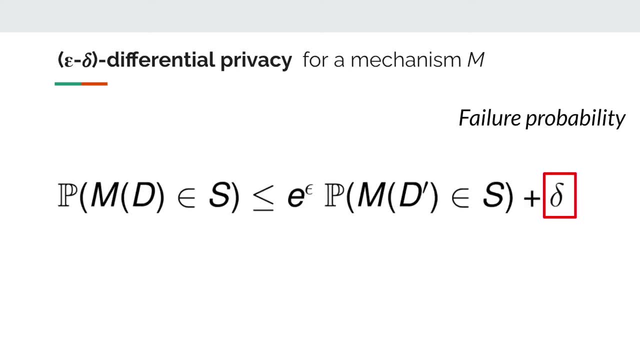 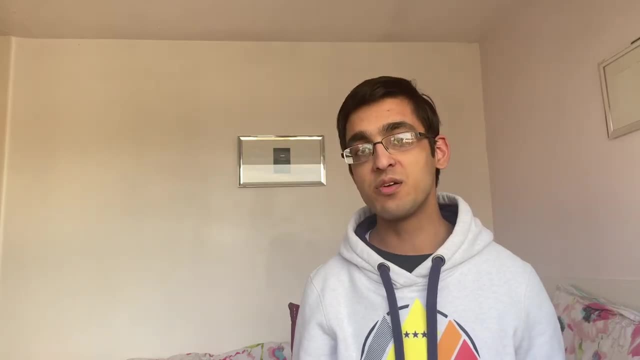 So we relax this definition slightly. so if we get epsilon, delta, differential privacy, where delta is this small failure probability? If we plot the privacy loss as a distribution, you can think of this as bounding the tail of the distribution In order to get these differential privacy guarantees. 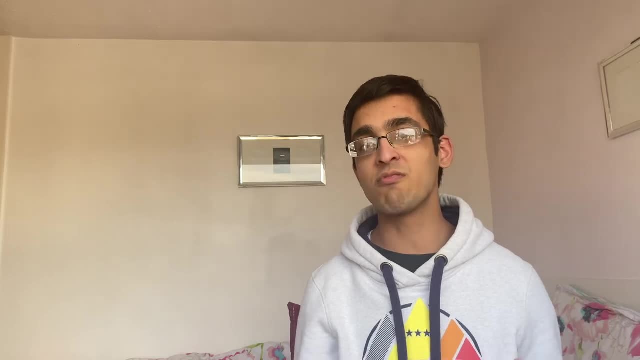 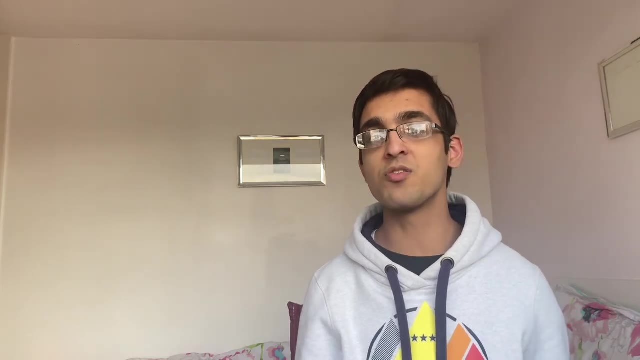 we typically add noise to our algorithm and this induces some form of randomness that helps us preserve privacy. We then statistically analyze this randomized algorithm to prove bounds on the maximum privacy loss. One technique we saw in the previous video explaining DPSGD is the moments accounted. 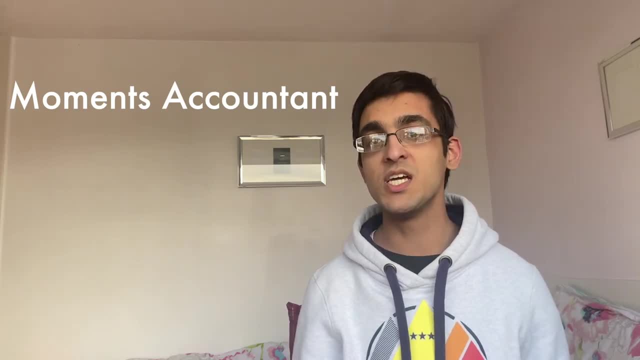 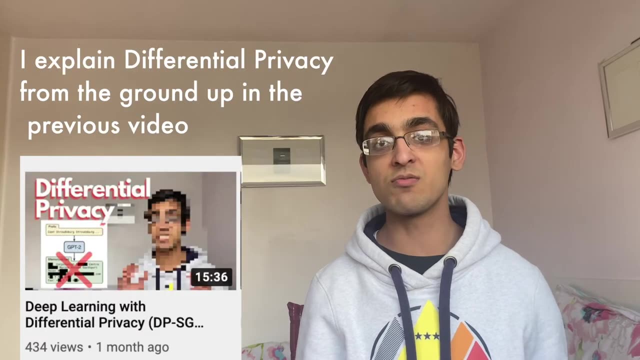 techniques, which takes our privacy loss distribution and derives a set of bounds based on the moments of this distribution, and I'll have the video linked below if you want to go recap that. With that out of the way, I'd like to give some intuition behind Pate. 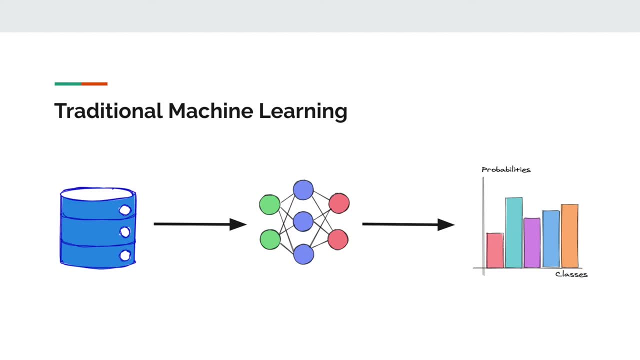 The setup for traditional machine learning is as follows. We train and model on some data and then predict some outcomes To ensure differential privacy. we need to add noise somewhere in this process to ensure the outcomes don't reveal too much about the private data. the model was trained on With DPSGD. we added noise during the training process. This meant that the 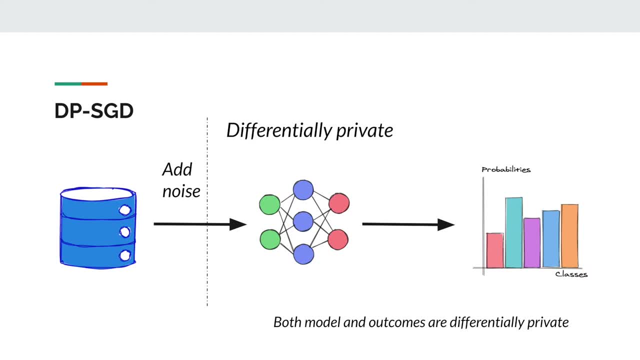 model itself is differentially private, so we're free to query its output however we like, but we trade off accuracy for privacy. as the gradient updates to our model are a bit noisier, How about if we added noise at a different stage of the process? What if we trained the model as normal? 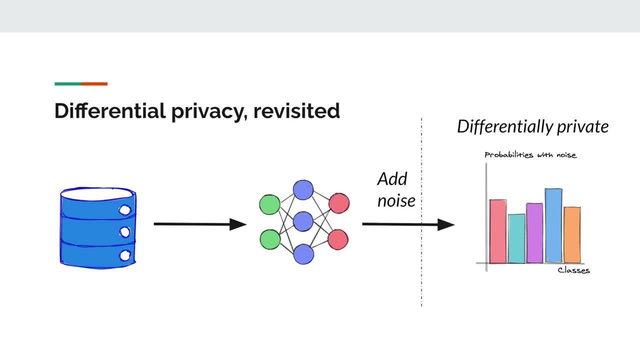 but instead added noise to the outcomes. Unfortunately, in our current setup, the noise needed for privacy would overpower the output and drastically reduce our accuracy. The issue here is that we're being heavy-handed with the noise we're adding. When our model outputs a prediction for a certain example, we're not. 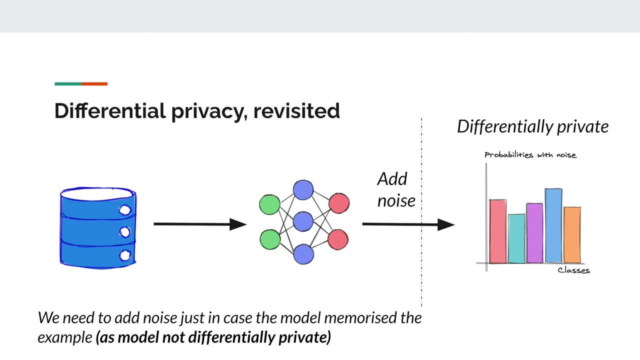 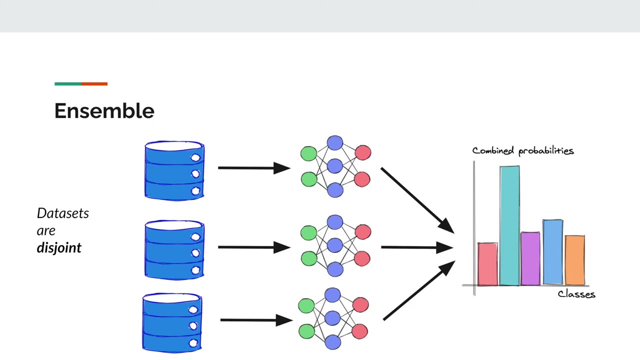 sure that's because the model memorized that example, or if it had learned a general trend. so we're having to add noise in order to preserve the privacy of that model. However, if instead we train an ensemble of models each trained independently on disjoint data set, then they can't all have memorized that. 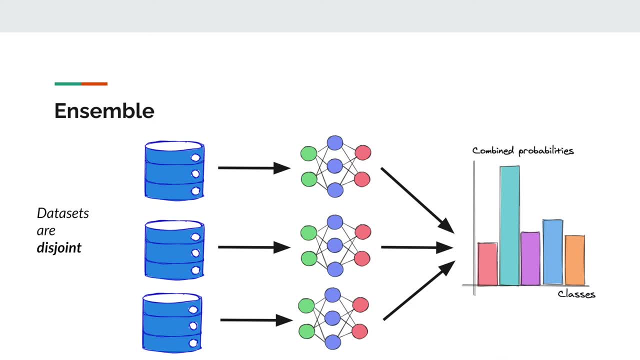 example. If they agree, it's more likely it's because of a common trend they've learnt rather than information specific to that example, and the more models we add, the more confident it's because of this common trend. This means we won't have to add as much noise because we're more. 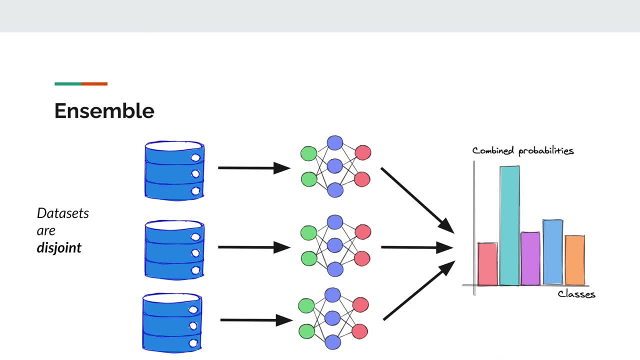 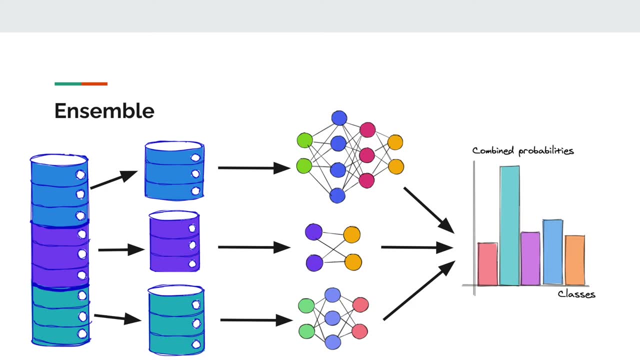 certain the privacy will be preserved. Going back to our original setup, we can get an ensemble of models by partitioning our data set into disjoint partitions and training models on each of them partition. The nice thing about this is that the models don't all have to be the same. they can be. 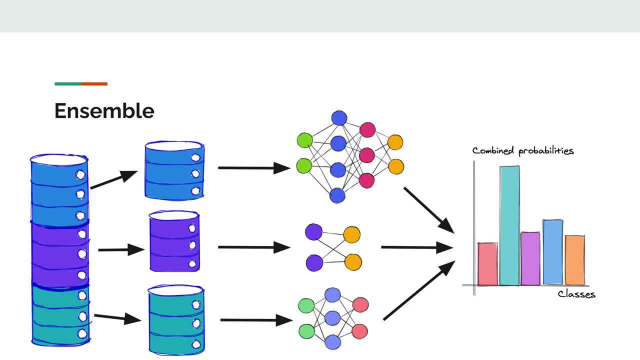 any classifier, You could have neural nets on one partition and logistic regression on another. In order to predict an outcome, say one of k classes, we aggregate the predictions of the ensemble of models. Each model contributes a vote as to which class it thinks it is, and we take the 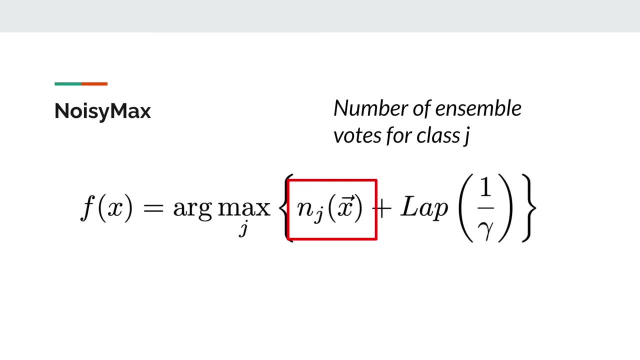 argmax, the most voted class. To guarantee differential privacy, we add noise to our votes so we can't tell what specific model voted, and this overall aggregation is called the noisy max operation In this equation. you can see the noise here is sampled from a Laplacian distribution with. 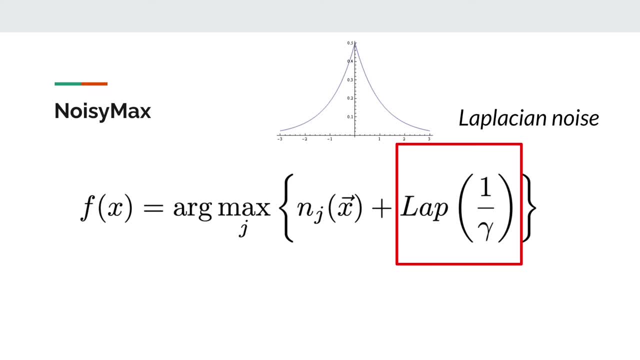 scale one over gamma Gamma. here is our privacy parameter. The smaller it is, the wider this Laplacian distribution gets, so the more noise we add, We can show that for a given gamma the noisy max operation is actually two gamma differently private. That is our privacy budget. epsilon equals. 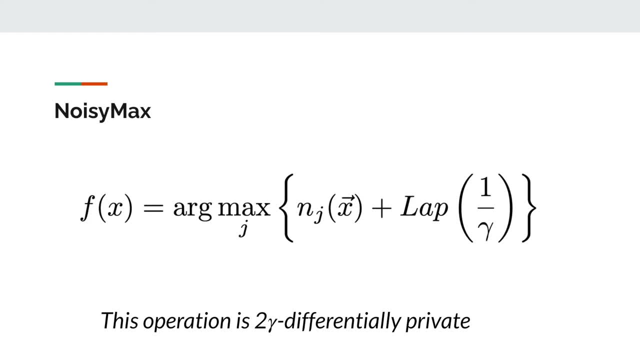 two Gamma and delta equals zero. The more models in our ensemble, the larger number of votes, which allows us to add more noise without affecting the consensus too much. So we can use a smaller gamma to get a smaller privacy budget. However, the more models we add, the smaller split of the data. 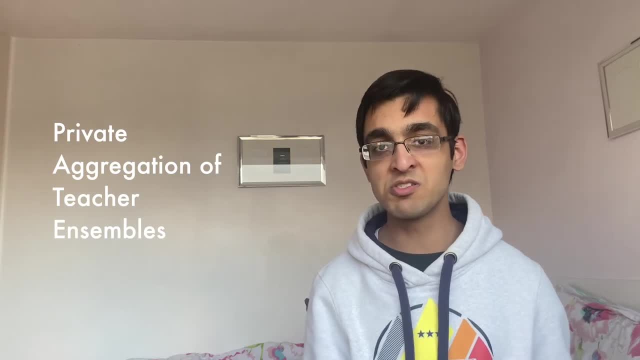 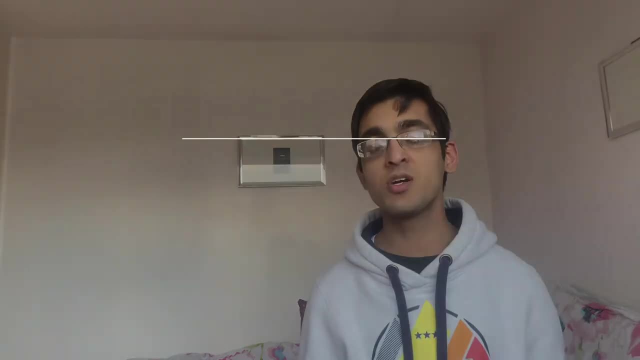 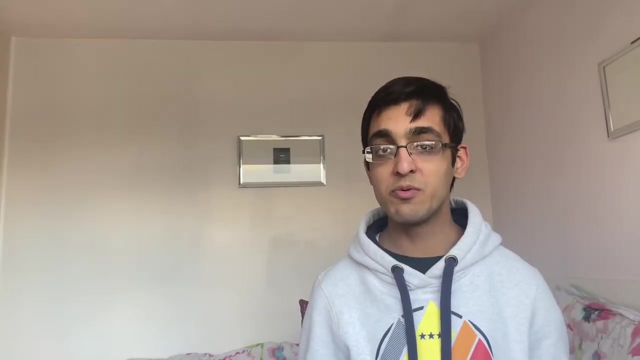 that each model gets Right. so we've introduced the ensemble and the private aggregation method. that is the noisy max. but there's one letter left in pate T. We can't deploy the model ensemble as is for a couple of reasons. First, every time we query this ensemble we leak a little. 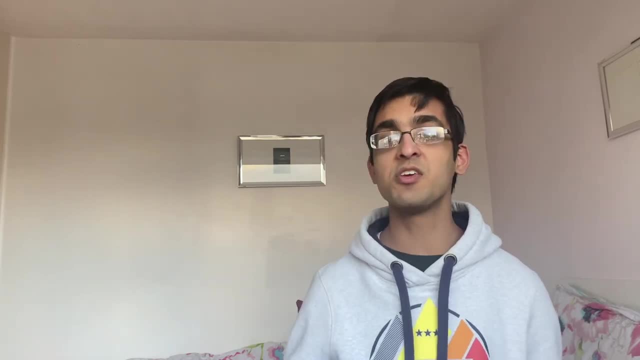 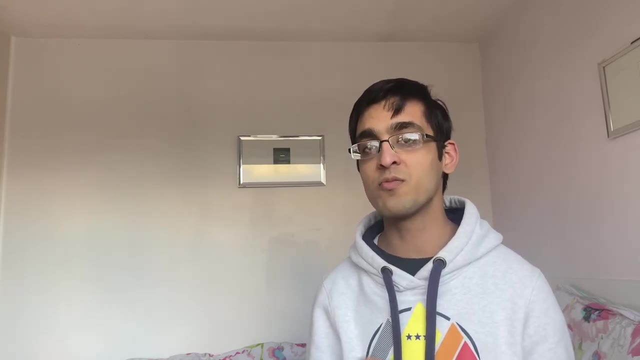 information about the data, and this privacy loss will continue to accumulate. Secondly, the model's weights encode information about the data they were trained on, so we wouldn't want this information to be made public. If we flash back to DPSGD, we didn't have this problem because we added noise. 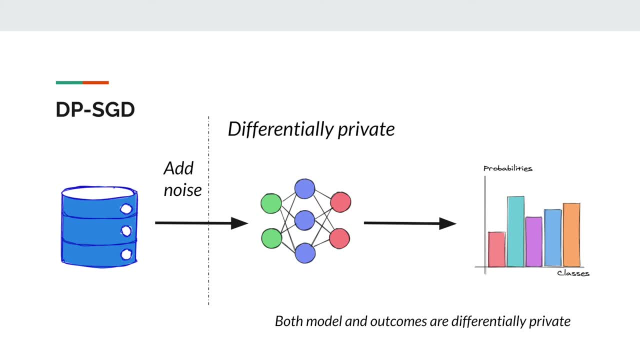 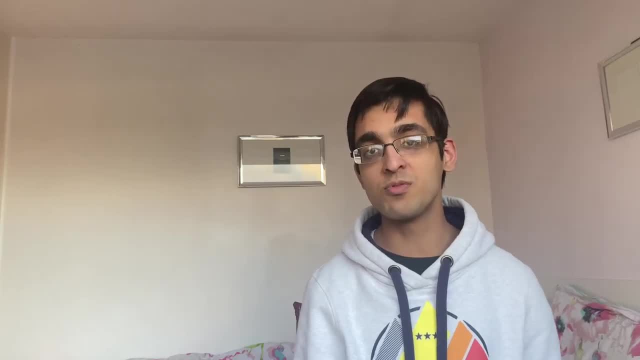 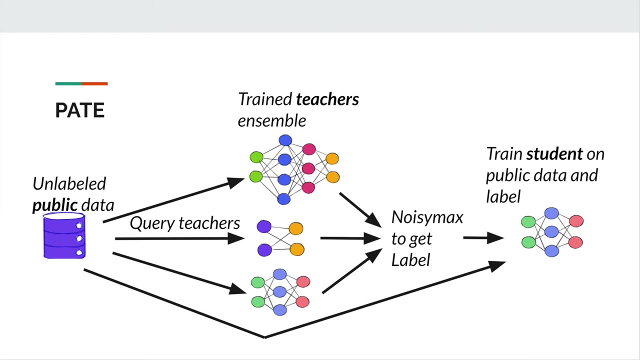 during the training process. so the model and the weights didn't encode private information, So the model itself was differentially private. Carrying over this idea, we can use our ensemble to noisily train a separate model that we deploy, which will be differentially private. In this setup we have some unlabeled public data that 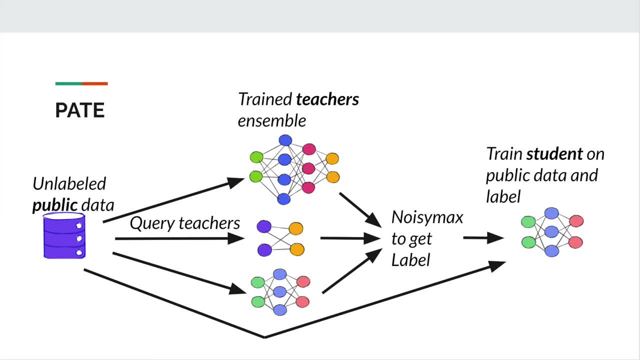 we'd like to train our deployed model on, and the role of the ensemble is to predict labels that the deployed model can use when training. We can think of the models and the ensembles as teacher models, whilst the deployed model is a student model, The noisy max operation used to 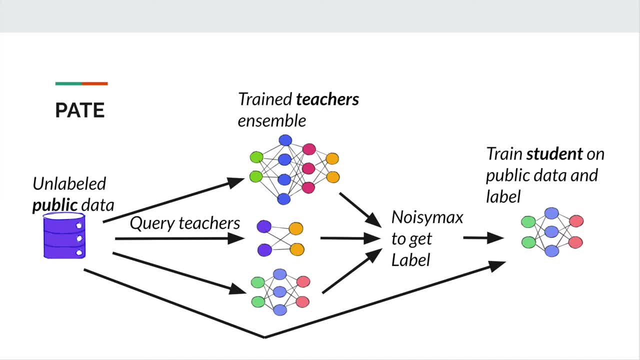 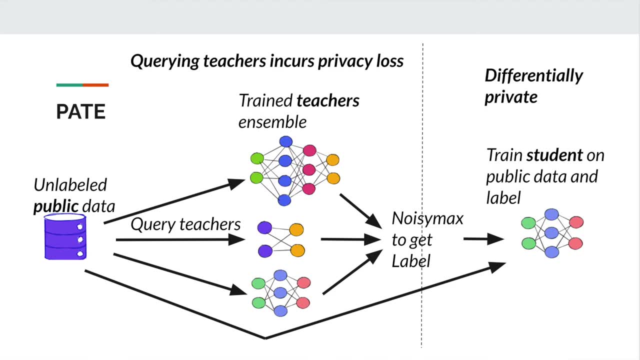 predict these labels adds the noise in the training process needed to train the model. Once training is complete, our privacy loss is now capped, as in deployment, we're not querying the teacher models At this point. we've covered the fundamentals of Pate, but there are a few more tricks. 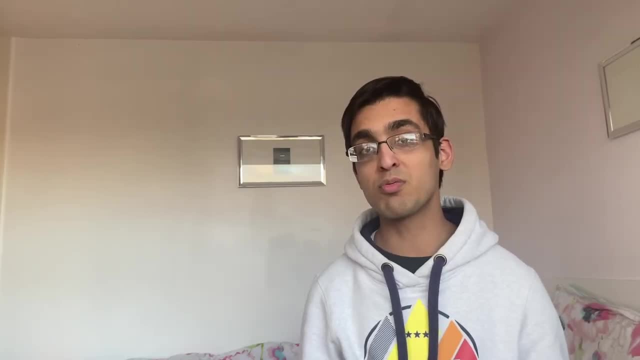 left in this paper and the next paper in order to improve the privacy guarantees we get with Pate. They fall into two camps. either we're trying to use more sophisticated privacy analysis to get a tighter bound for the same mechanism and therefore a lower privacy budget, or we're trying to improve. 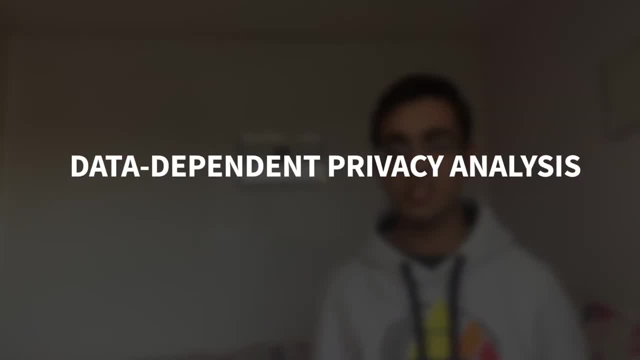 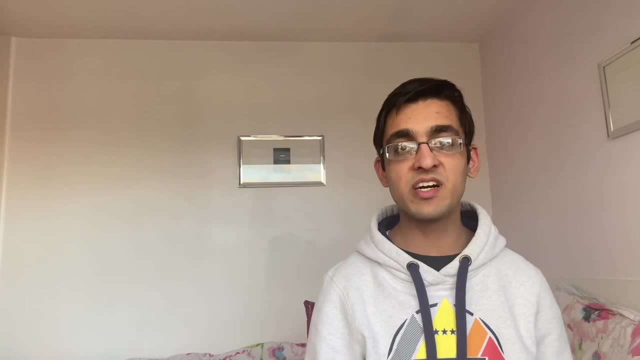 the mechanism itself. at the privacy analysis, Pate uses the moments accounting technique in order to derive the privacy guarantees. To get a smaller bound, we need tighter bounds for each of the moments. We can do this by incorporating properties of the training data into our analysis. 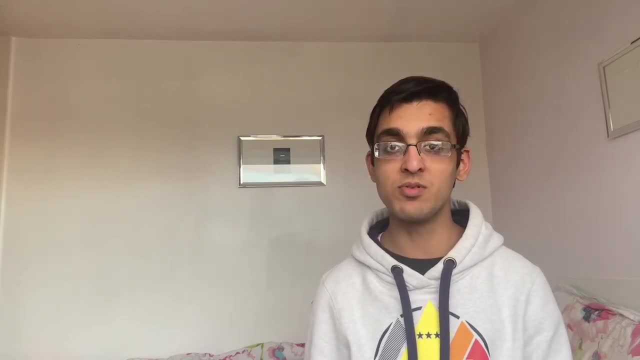 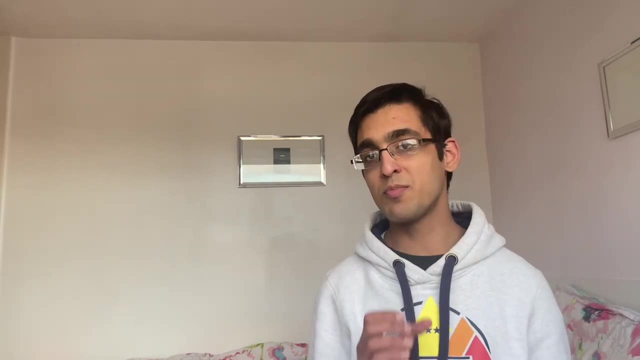 If the models in the ensemble agree really strongly on a particular example, then it's less likely that we've memorized the example and so the privacy loss for that example will be much lower. The details of what the bounds themselves are aren't too important, it's just this idea of 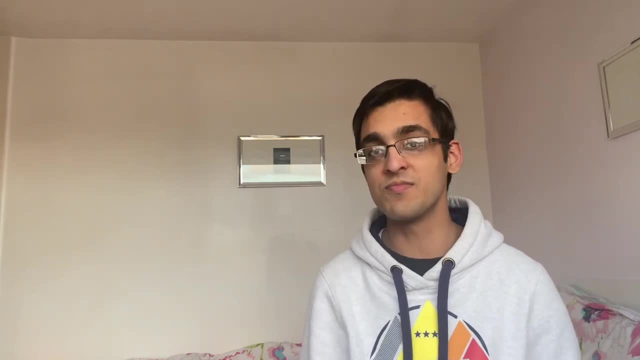 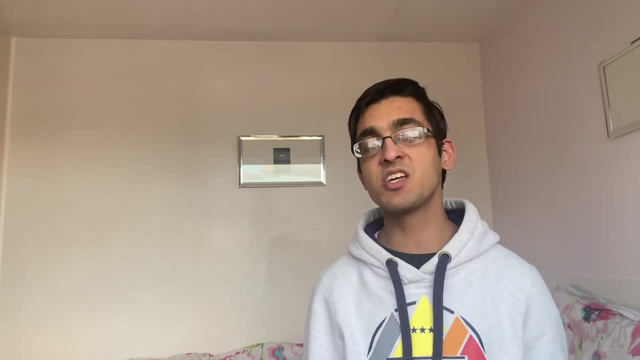 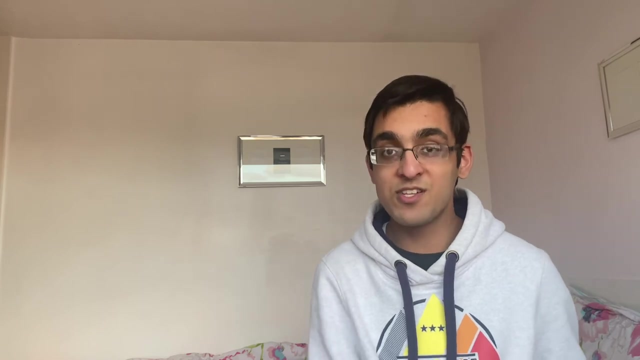 incorporating our data into analysis. that's important here. However, now that we've incorporated information about our data into our privacy bounds and therefore our privacy budget, releasing our privacy budget would actually reveal information about the training data. Therefore, in a somewhat meta twist, we apply differential privacy to the privacy budget. 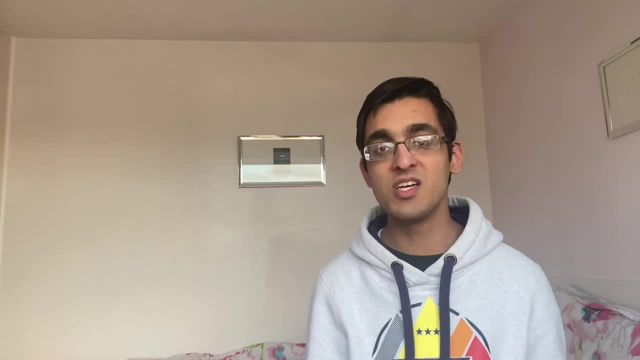 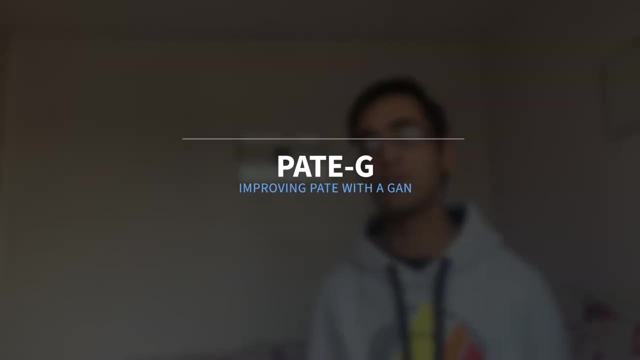 itself. that is, we add noise proportional to the moments to ensure the budget doesn't reveal information about the data. Kind of crazy, if you ask me. Taking the second approach of improving the mechanism itself, we know that every time we query our teachers for a label during the 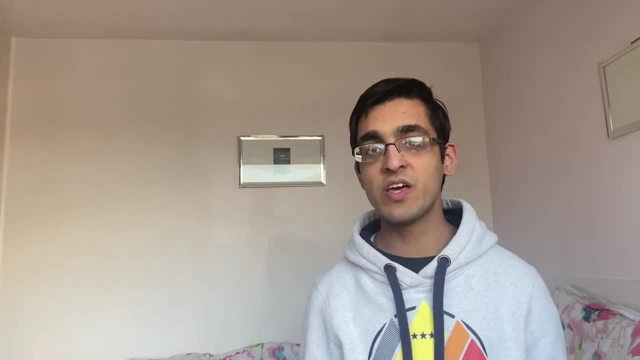 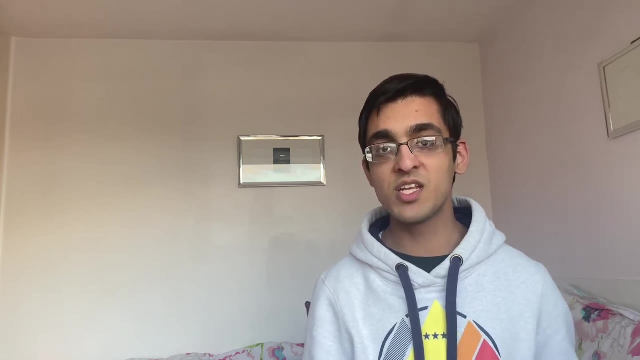 training process, we incur a privacy loss. Therefore, we'd like to reduce the number of queries during the training process. Other than training the student from scratch using the teacher's labels, we can instead pre-train it in an unsupervised fashion by setting up a GAN In this GAN. 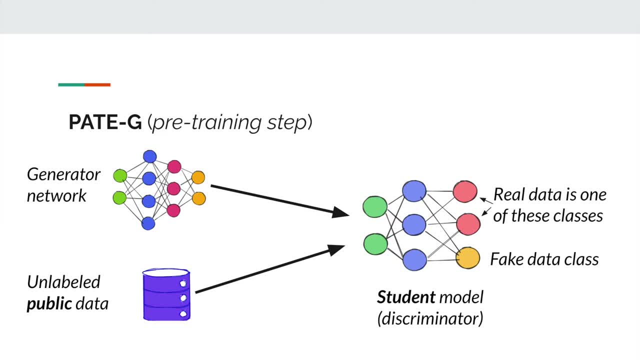 this gender of adversarial network, the student plays all the discriminator. Remember, the role here is to predict whether the data is real or fake. Our student model is set up to predict one of K classes. so to adapt it to this pre-training task, we add a dummy class for fake data and we train the student to predict one of the K classes. 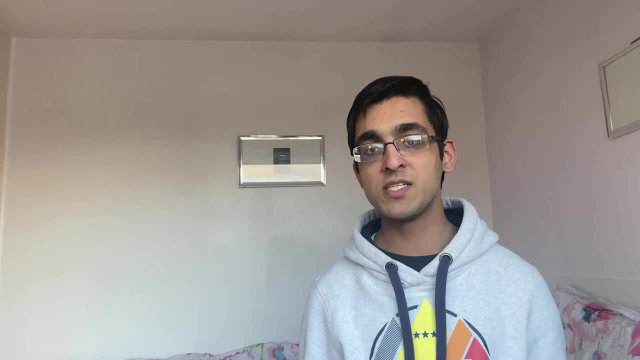 if it's real data and the dummy class if it's fake data. By doing this, the student effectively learns to extract features about the unlabeled public data, so that when we do try to label this with the teacher, it's only a process of fine-tuning the final classification layers. 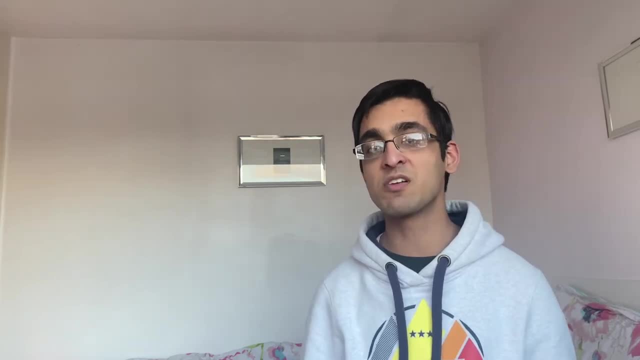 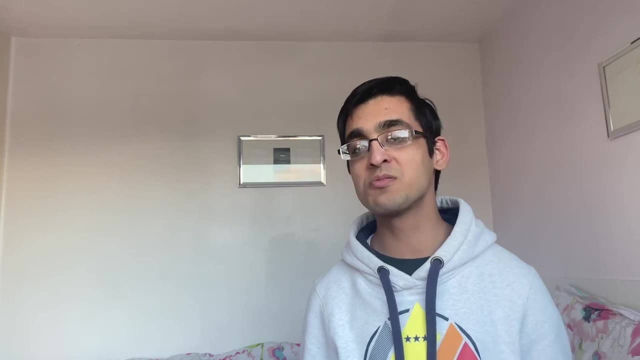 so it's much quicker to converge. When it comes to deployment, we can throw away the generator part of the GAN along with the teacher ensemble and just deploy the student Right. a quick pause before we tackle the second paper, which is enough time for you to hit that. 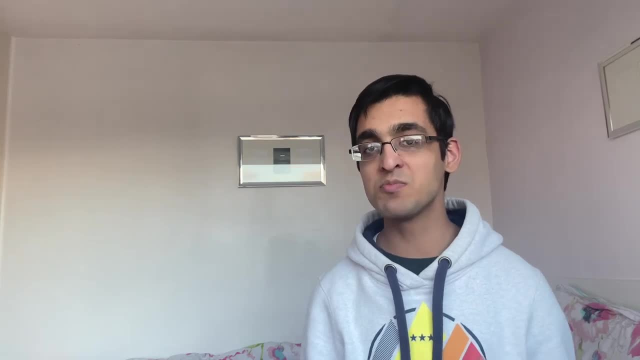 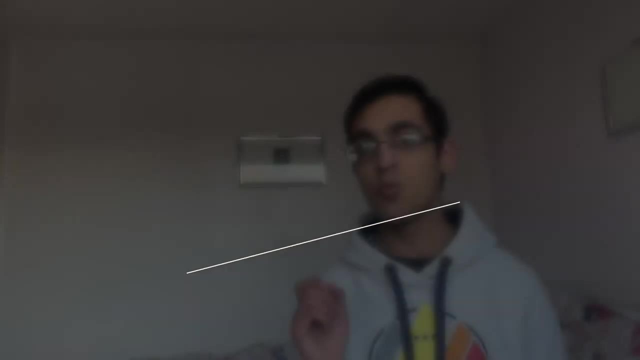 like button if you're enjoying this video. It's quick and easy and it helps small channels out, like mine, with the YouTube algorithm. The second paper looks to improve Pate's privacy guarantees by focusing on one part of Pate- the NoisyMax aggregation mechanism. 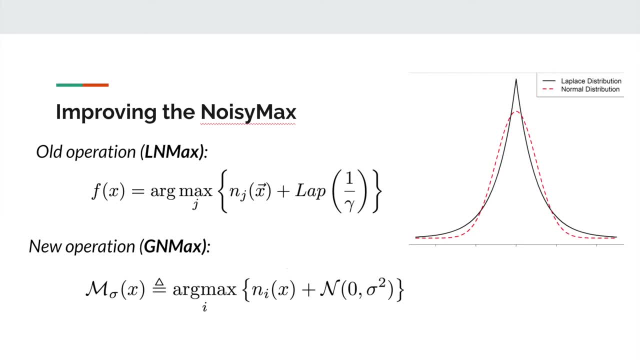 First we change the noise distribution from a Laplacian distribution to a Gaussian distribution. As it's more concentrated, the tails decay faster. in the Gaussian distribution We call this the Gaussian NoisyMax, or the GMX for short, and the previous one would be called 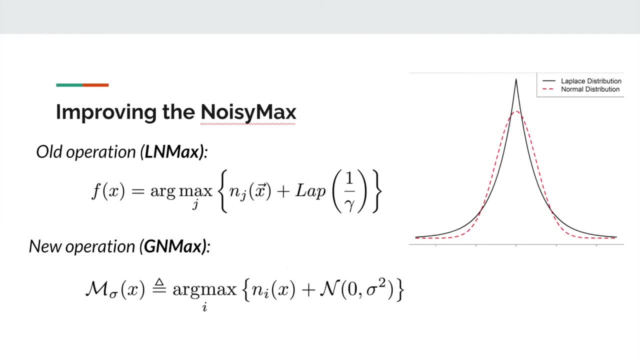 the Laplacian NoisyMax or LNMax. Changing the noise distribution means we need to re-analyse the NoisyMax differential privacy guarantees. It turns out that epsilon delta differential privacy isn't well suited to analysing Gaussian noise and a better approach. 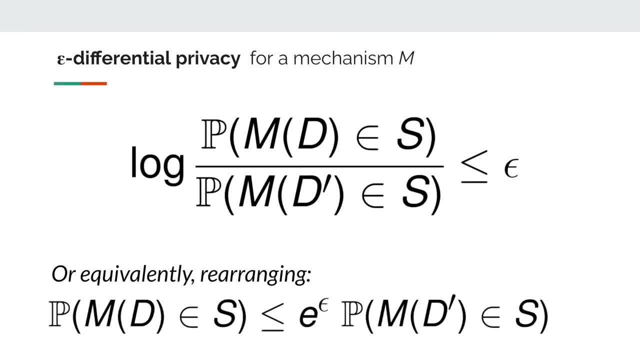 is Renyi differential privacy. Our original definition of differential privacy was epsilon differential privacy, but we bounded the max amount. the log of the two ratios of the outputs could vary by this privacy budget epsilon. This definition is commonly referred to as pure differential privacy, but we loosened it by adding a failure probability delta. Renyi differential. 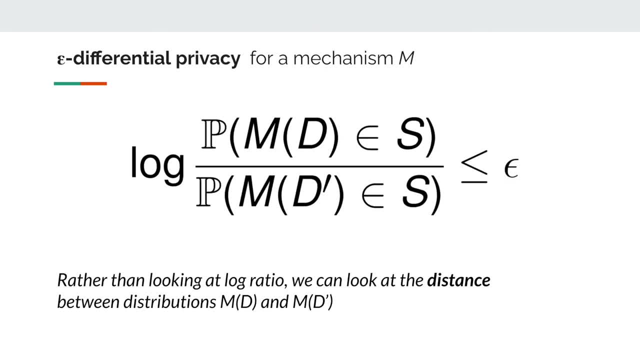 privacy is another way of relaxing this pure differential privacy guarantee. Instead of looking at the log ratio of the properties, we look at the distance between the two output distributions. Specifically- and this is where the name comes from- we use the Renyi divergence to measure the 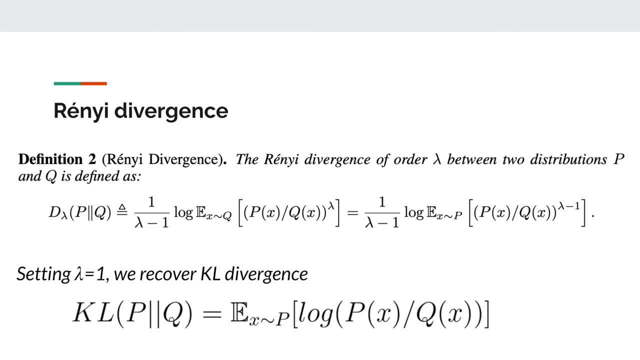 distance between the two distributions. You don't need to read too much into the formula, you just need to accept this as a distance metric that we're using. that is parameterised by some lambda Setting. lambda equals one. we recover KL divergence, which you might have seen when looking at. 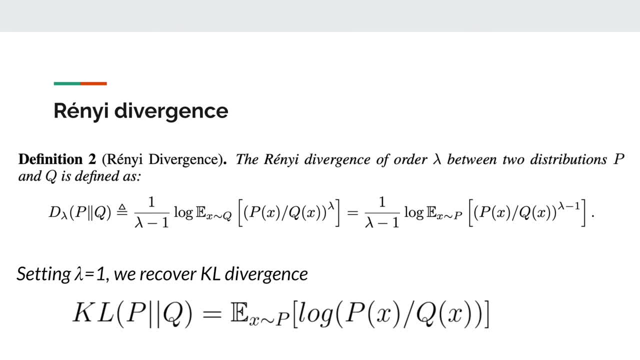 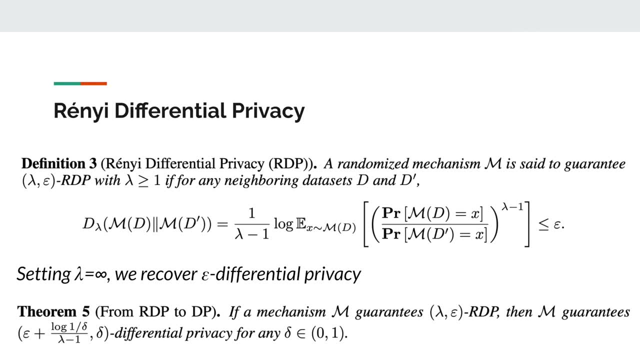 variational auto-encoders, or RDP for short, is parameterized by both lambda and our privacy budget, epsilon, and states that the maximum distance for any data sets of D and D prime is bounded by our budget epsilon. We can go between definitions of differential privacy. Setting lambda equals infinity, we get. 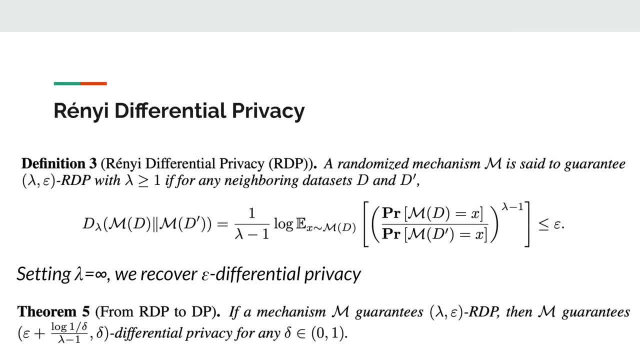 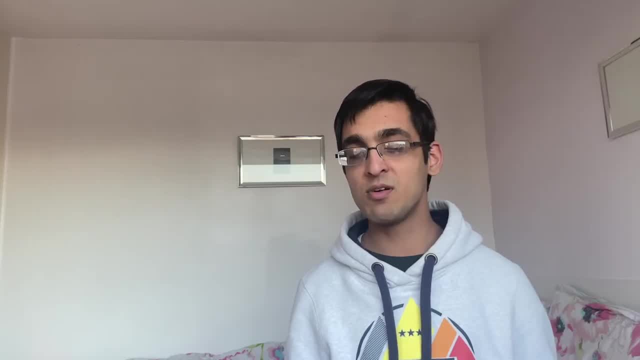 epsilon differential privacy and likewise there is a formula to convert RDP to our epsilon delta differential privacy. I'll drop a link to a talk by Ilya Mironov, the author who coined differential privacy, if you're interested in learning more. but suffice to say this definition of differential. 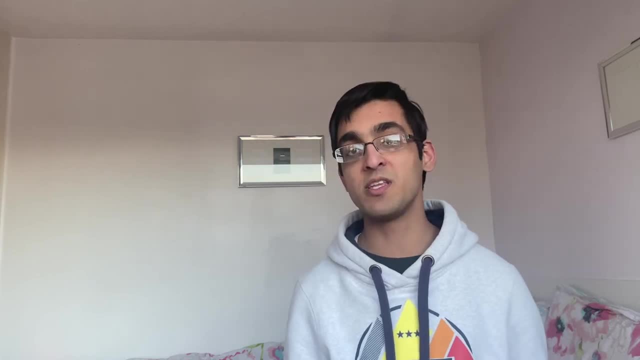 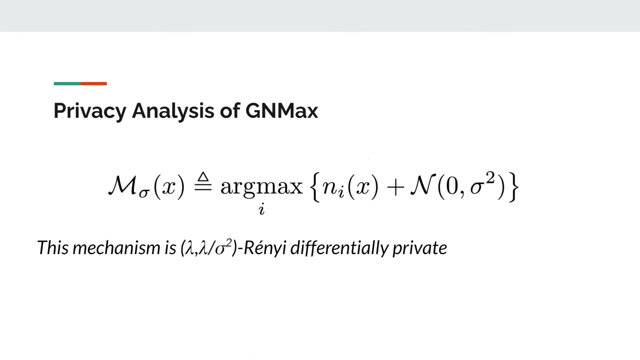 privacy satisfies all our properties that we talked about in the previous video. like composition With RDP, we can prove a privacy guarantee for GNmax. If we add noise with variance sigma squared, then the GNmax mechanism satisfies lambda over sigma squared RDP. You can see that the 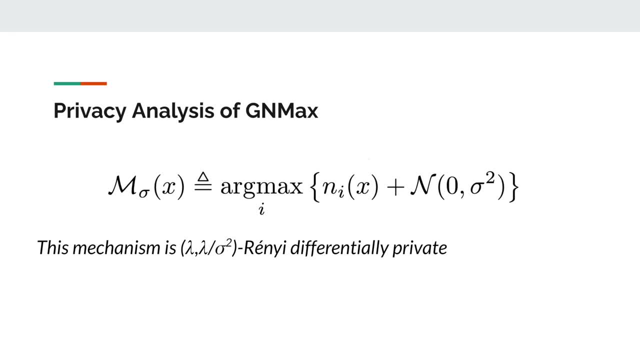 privacy budget here is equal to the value of RDP over sigma squared. So if we add noise with variance, it's inversely proportional to the variance of the noise, which intuitively makes sense. As in the first paper, doing a data dependent analysis gets you a tighter bound. only this time. 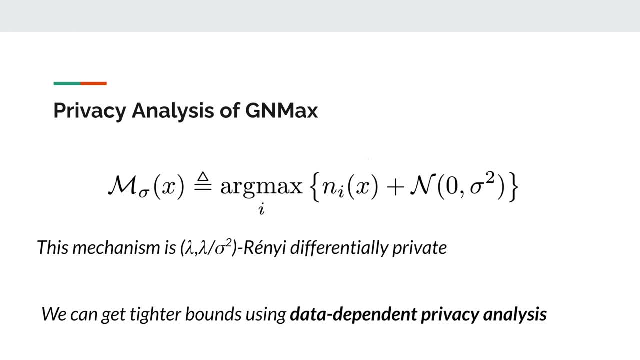 the maths derivations are even messier, so much so that it gets relegated to the appendix of the paper. The maths works out the same Queries where the teachers agree more on have a smaller privacy loss. The second part of the paper tries to improve the aggregation mechanism by only returning an answer. 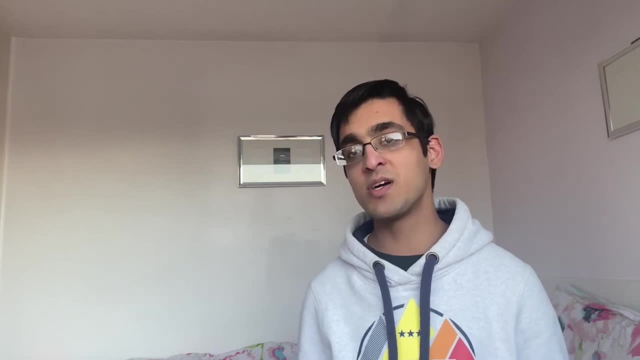 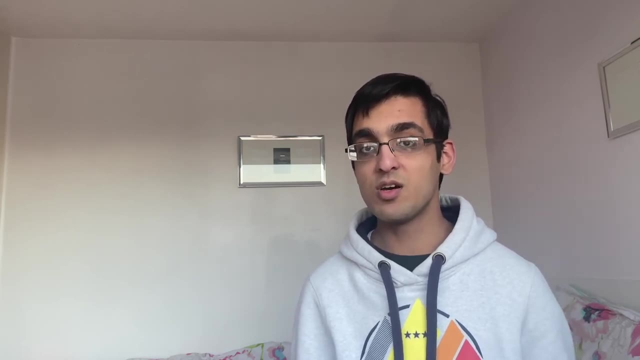 from the teachers if it would be useful. There are two scenarios: where an answer says no and it might not be useful to return an answer When the teachers aren't confident themselves about the correct label, and when the student already knows the answer and is confident. 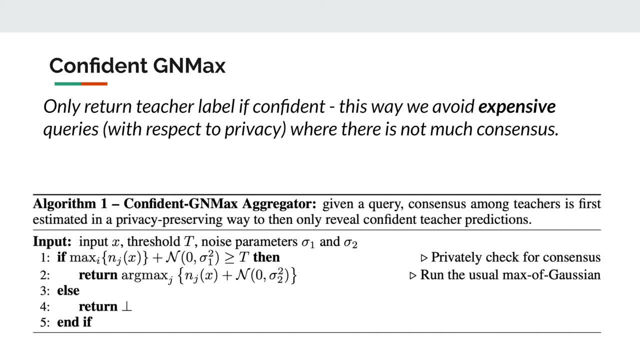 As the name might suggest, the confident GNmax aggregator only returns the noisey max of the label, the, if there's sufficient consensus among the teachers, That is, the highest vote is above a threshold, t, which is typically 60-80% of the teachers. if not, we don't return the label. 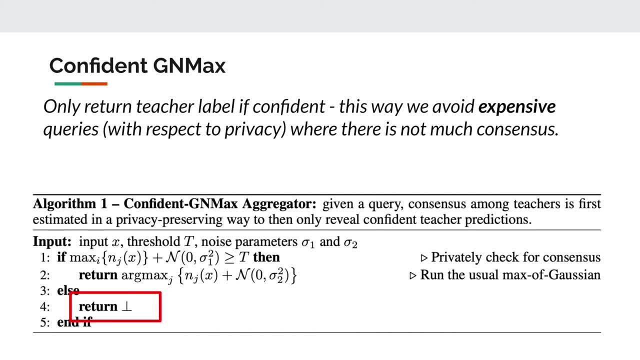 But since the decision whether to return a label or not reveals- well, you guessed it- information about the underlying data, we add noise to this thresholding operation Because we're running this check every query, and since we don't need as high fidelity to determine the threshold versus. 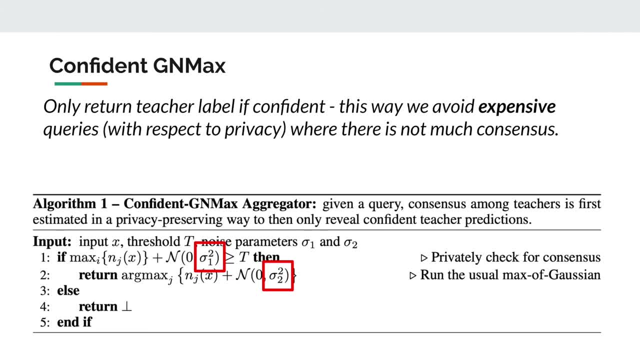 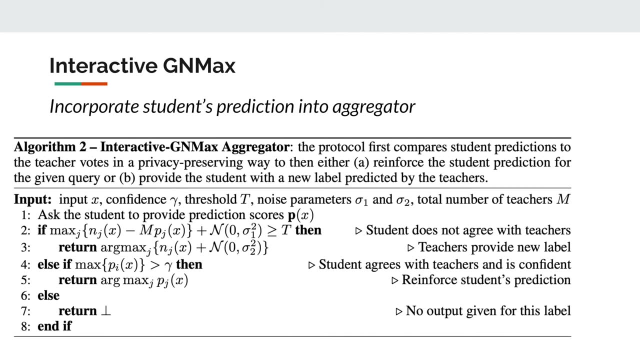 determining an individual class, we typically add much more noise. Sigma 1 is higher than sigma 2.. This extra noise is okay, because all that would happen is you discard queries. that actually has drawn consensus. We can take it a step further with the interactive GNmax aggregator. Not only 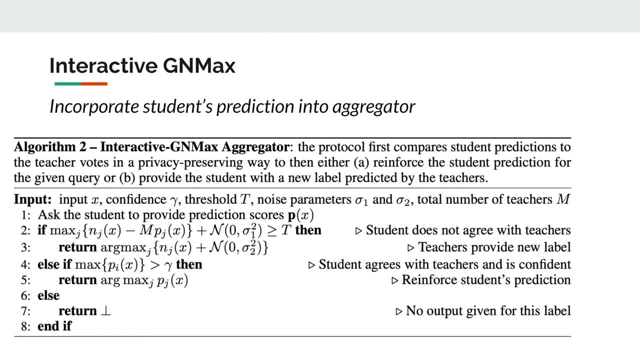 do we look at whether the teachers are confident, but also if the student is confident knows the answer. First we check whether or not the student agrees with the teacher, because there's no point in reinforcing the prediction if it's incorrect To compare against teachers votes. we take the. 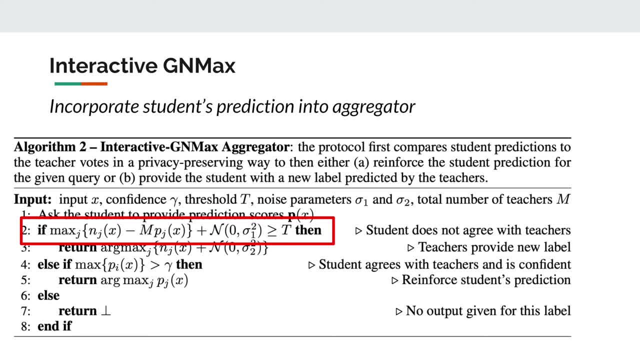 prediction probability, pj, and scale it up by the number of teachers, n, to get an effective average number of votes the student would have given. We subtract this from the number of votes the teachers gave for that class j. If the student agrees with teachers, then the 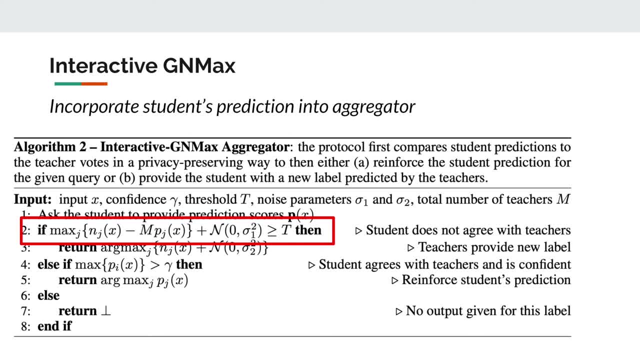 number of votes given by the teachers. nj and m times pj will cancel out for each class. However, if the student disagrees, then for the teacher selected class, nj will be pretty large but pj will be quite small. Note that if the teachers aren't confident, then nj will be less. 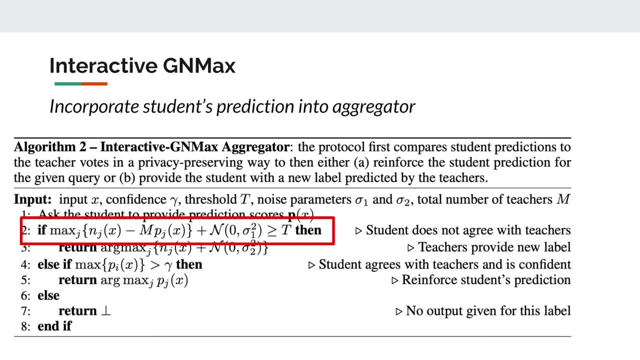 than the threshold. So if the teacher agrees with the teacher's decision, then the number of votes t that we need, and so nj minus mpj will also be less than the threshold. so the teachers won't provide a new label if they aren't confident. so this if statement on line two means that the 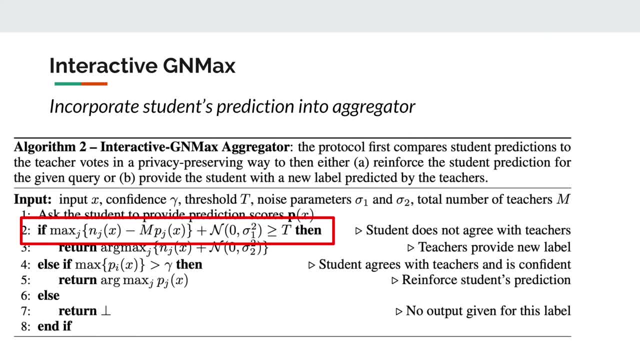 teachers will only provide a label if the teachers are confident and the student disagrees with the teacher. therefore, in the else condition we know that the student agrees with the teachers, so we check if it's confident or not. so if it's above a threshold gamma and if so, we just reinforce the 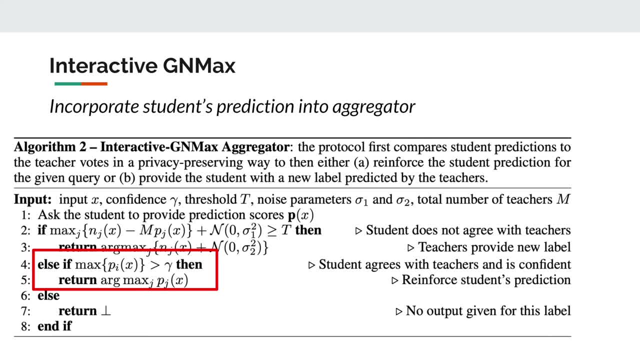 student prediction by returning its most positive class, the argmax. and if neither of these conditions hold, then we don't return a label, because the teacher isn't confident and the student doesn't agree with the teacher. now you might be asking yourself why, on line two, do we add noise to our 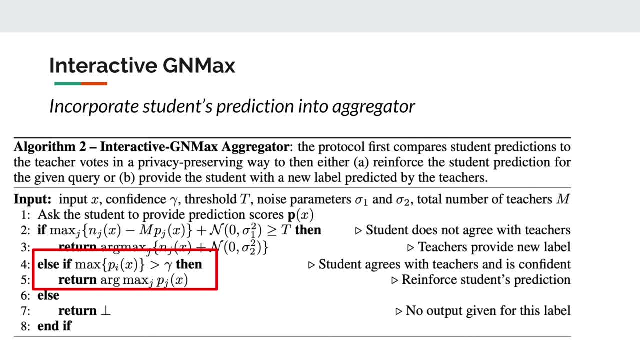 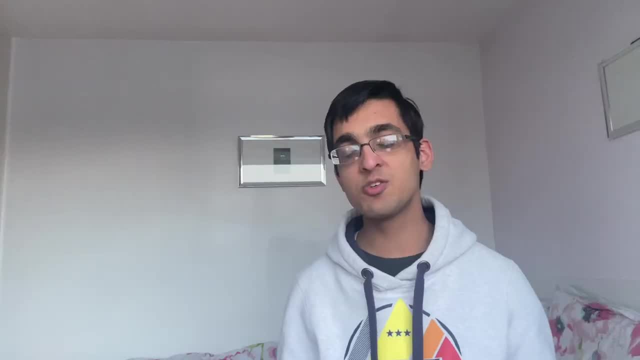 thresholding check, but we don't do the same for line four. for our student threshold gamma, we know that the student is trained in a differentially private manner, so the outputs of the student wouldn't reveal additional information. therefore, we don't need to add noise to preserve privacy when training the student with this. 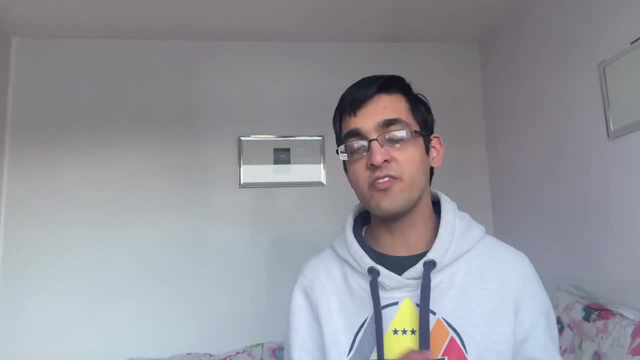 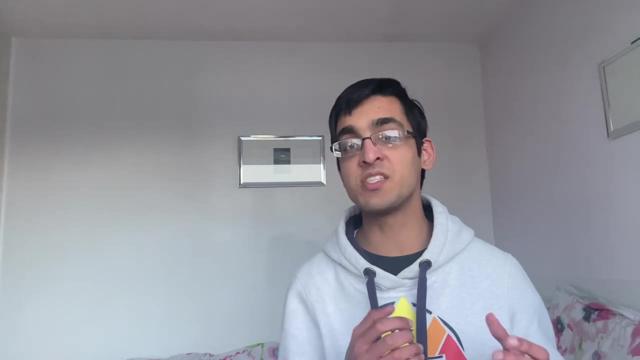 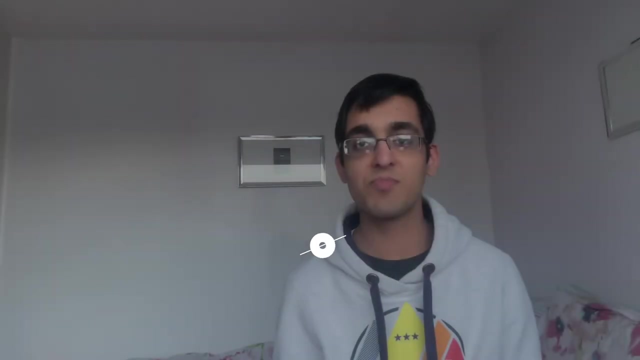 improved version of paté. you might start off by only using the confident aggregator and then, once the student has become sufficiently accurate, you can start incorporating its predictions using the interactive gm max aggregator. to wrap up this video, i want to talk about the relationship between privacy and accuracy with dpsgd. in the previous video we found those, this tension between privacy. 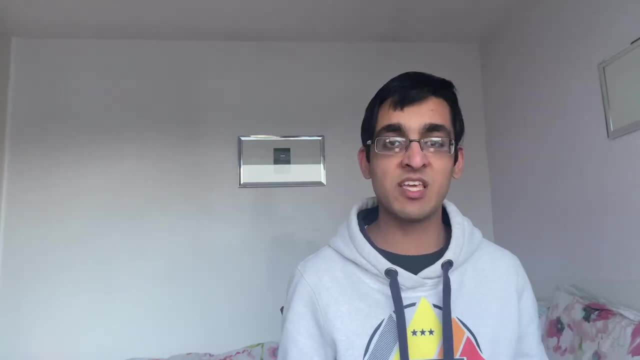 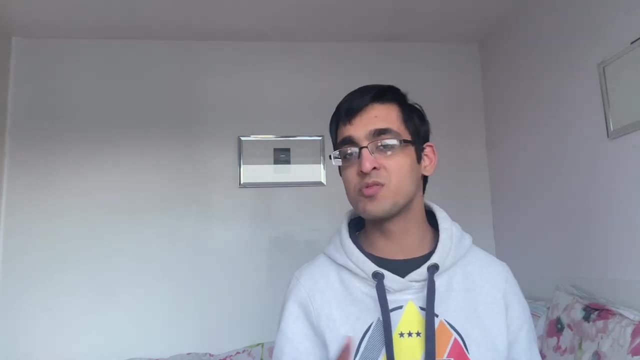 noise, increased privacy, but at the detriment of accuracy, as the grading updates were much noisier, so the model couldn't learn a better representation in pate. this noisy max added to the training of the student model would also similarly degrade performance. however, in the follow-up paper.